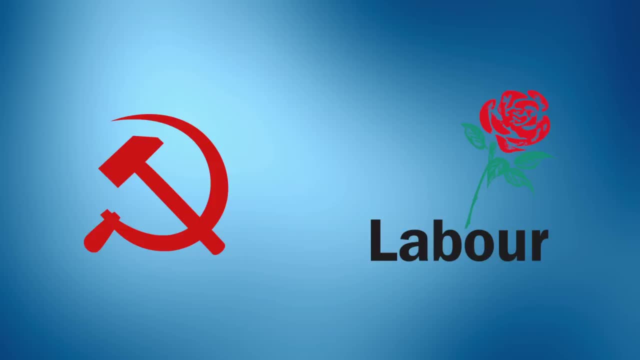 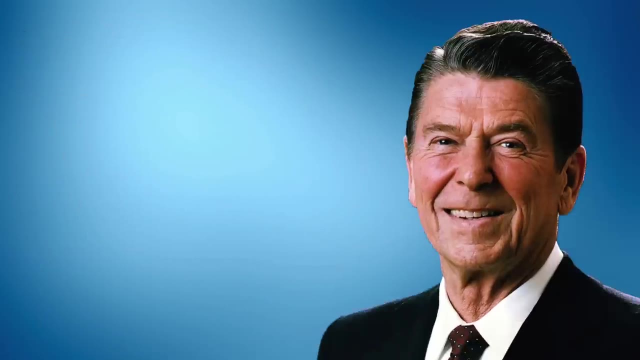 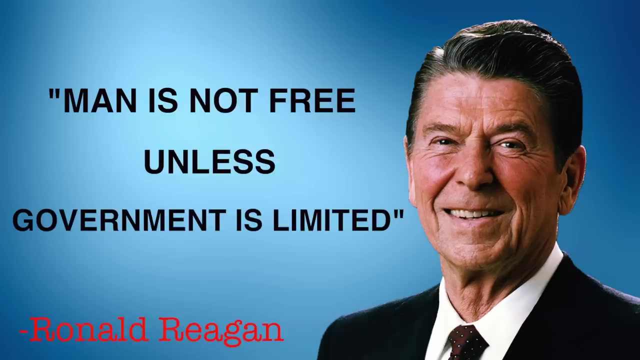 wanting complete control over all aspects of the economy, whereas the centre-left want only moderate intervention. The right believe that a level of social inequality is inevitable and think that the government should have a limited role in people's lives and business. This is as the right believes that preserving personal freedom should be the government's. 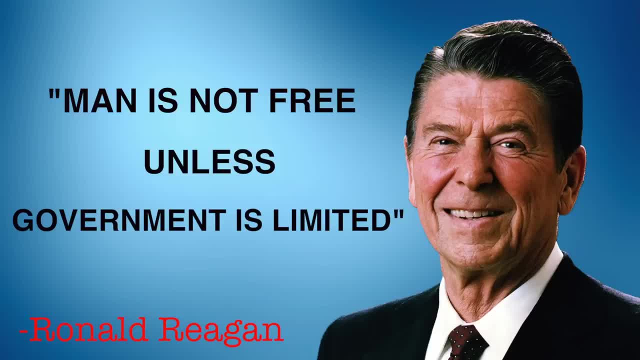 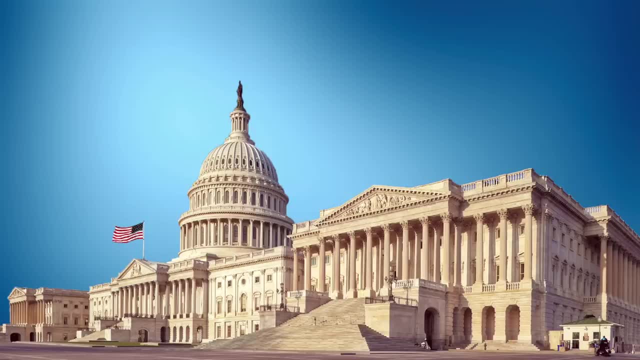 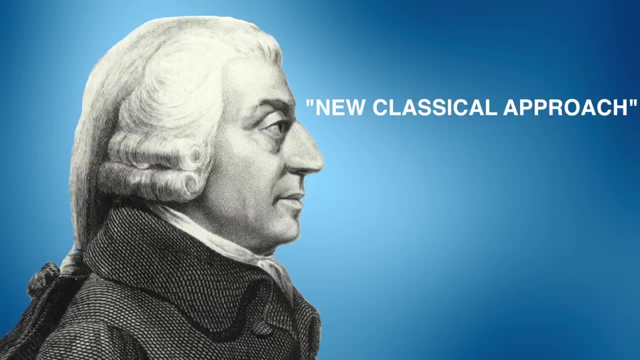 main goal and should not impose too many rules on people's lives. The right also tend to hold more traditional and religious attitudes than the left, often opposing things. those on the left support such as same-sex marriage and women's right to abortion. Economically, the right can often be seen using the new classical approach, which includes 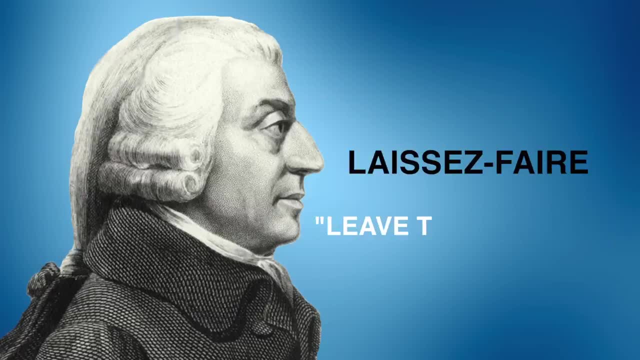 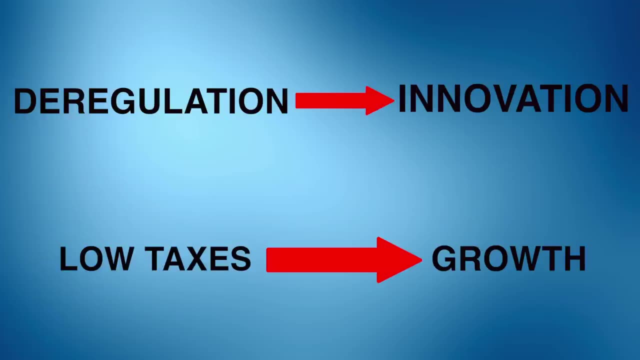 having a laissez-faire policy. This roughly translates to leave things alone and means less regulation to increase innovation and lower taxes to increase growth. In short, the right views government interference in business as a bad thing and thinks that the market prospers best. 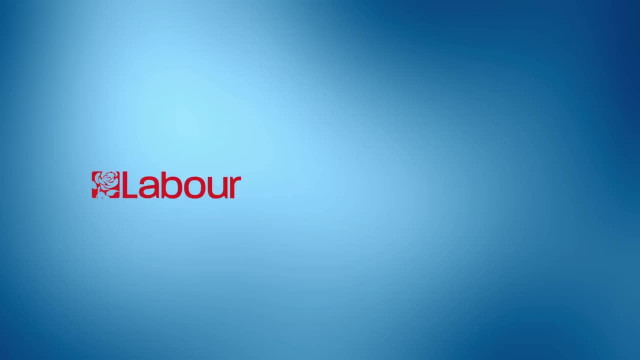 Parties on the left include Labour, the Greens and the Democratic Party, while those on the right include the Republicans, Conservatives and the UK Independence Party. There is also a centre-ground where parties like the Liberal Democrats lie. These parties hold views from. 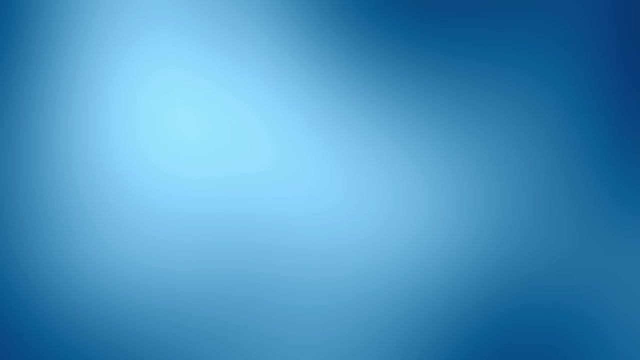 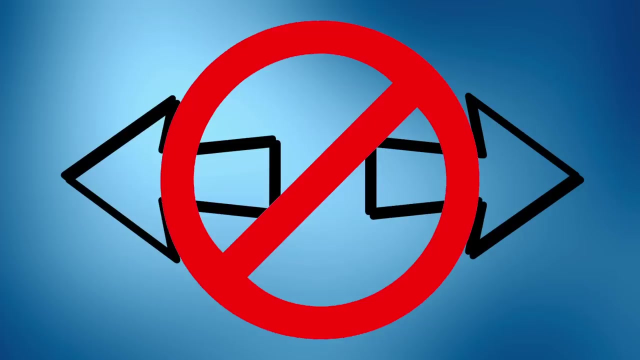 both the left and the right. This all being said, the use of left and right to describe modern political parties is not always accurate. There are actually many different political spectrums that can be used to judge how far left and right are different. 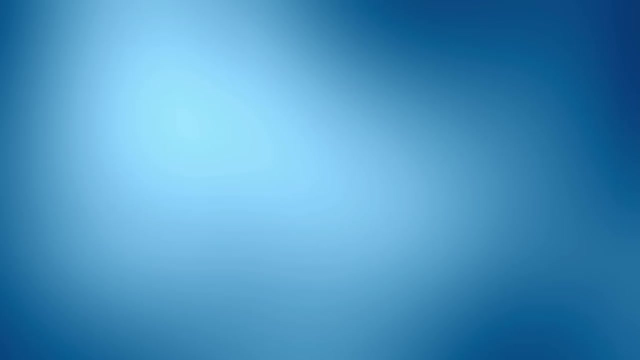 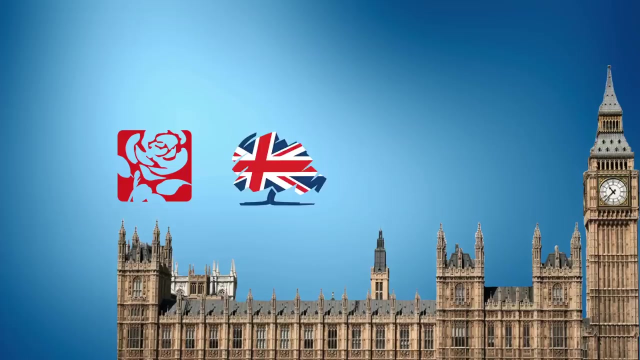 Parties often judge themselves based on other current political parties. In this regard, Labour is often seen to be on the left and Conservatives are often seen to be on the right. In actual fact, lots of Labour policy actually places it in the centre or right of the political 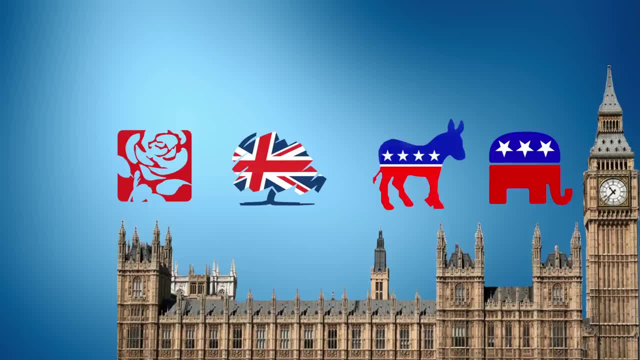 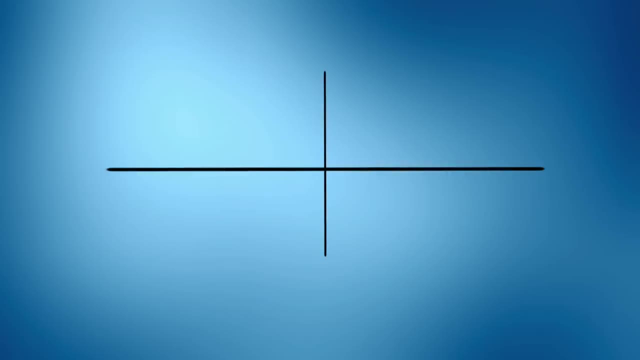 spectrum. The same is true in America, where both the Democrats and Republicans are on the right of the spectrum in political terms, even if the Democrats are sometimes seen as having more left-wing values. The political spectrum is also not just two-dimensional. Within both the left and right, there are people. 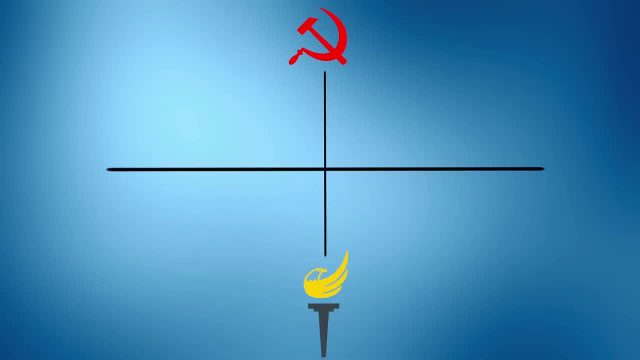 who hold authoritarian and libertarian views. Authoritarians wish for greater government interference and libertarians want the opposite. As previously stated, the left tend to be authoritarian and the right tend to be libertarian, but this is not always the case. We are often.